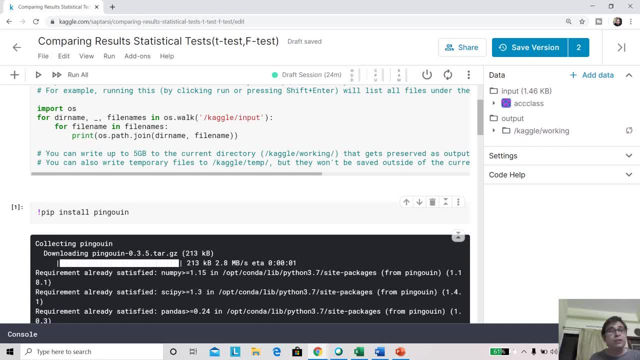 So the question might seem very simple. So you will understand why it is complicated in a little while. And then we will also find the answer through a hands-on posted in a Jupyter notebook in the Kaggle environment. So this will be available as a public notebook, available in the video description. 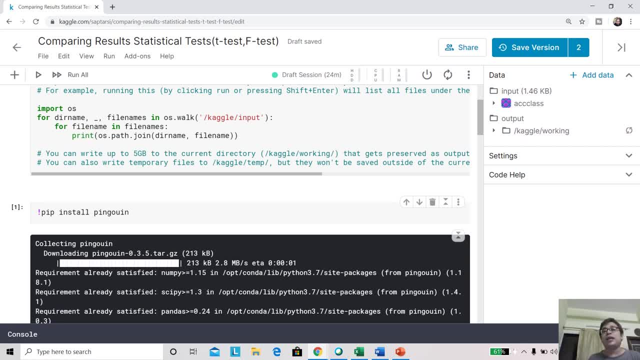 You can run, change suit for your particular case and get your results. So you need a library for this Pinguin, which we have installed here, And then we are going to import our normal libraries- Pandas, then SkypeP for 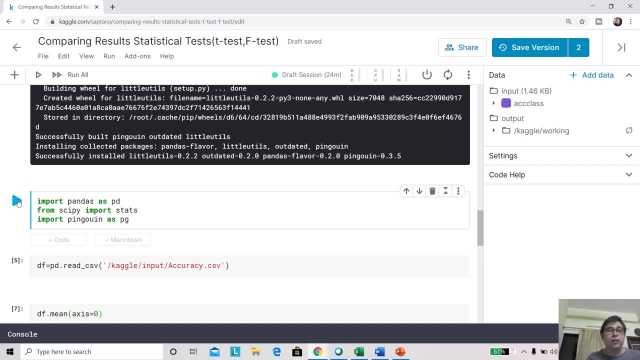 So we have our stats and this just installed library is Pinguin. Now we've already prepared the set, right, So let me run this, and when I will show you the dataset, you will understand what we mean by that. the dataset is already set up. 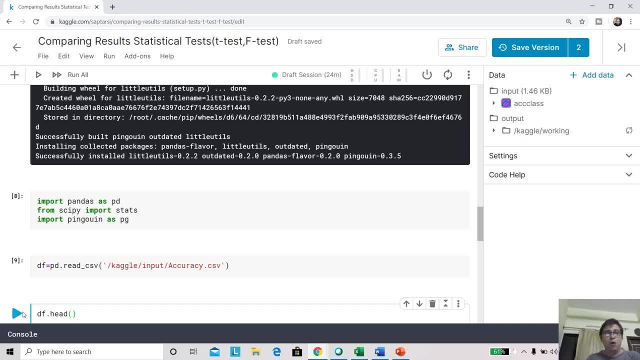 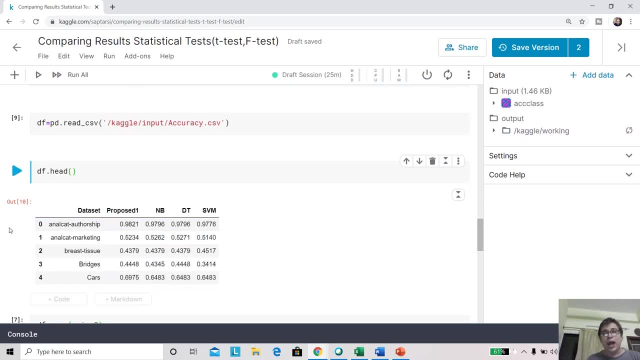 So let's just run it and see how this looks like. So you know, you see that actually each row has one dataset And this is a proposed algorithm. And these are three competitive algorithms, maybe name-based decision-true and SGN. okay. 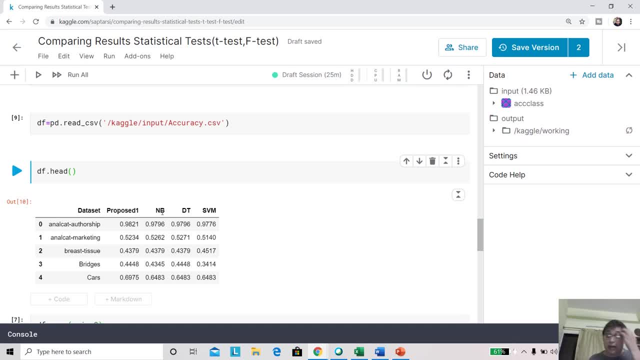 So your question is, as I said, that is my proposed algorithm better than all these three algorithms? So one of the simple arguments can be that I can find the mean right. So I can simply find the mean of all these methods like this: 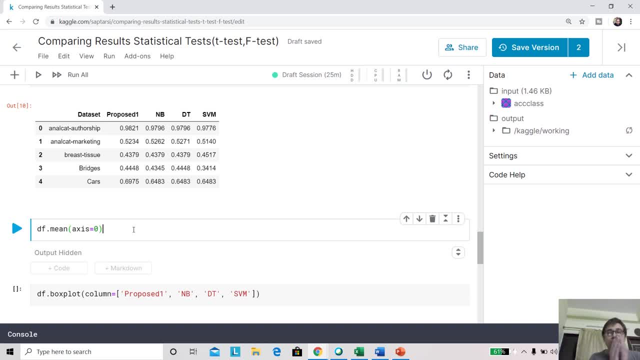 So you know, axis equal to zero gives us the mean of the columns, and axis equal to one gives us mean of the columns. So you know, axis equal to zero gives us the mean of the columns, and axis equal to one gives us mean of the columns. 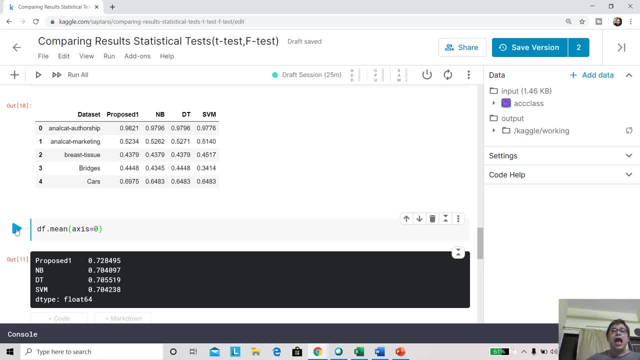 So you know, axis equal to zero gives us the mean of the columns and axis equal to one gives us mean of the columns. And you see that proposed has an average classification accuracy of 72.84, followed by 70.4, 70.55, 70.40. 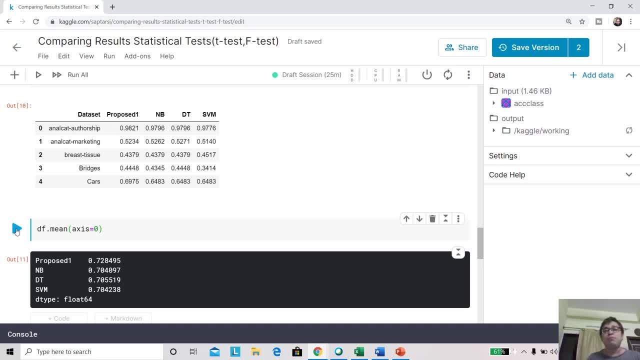 So you might be very tempted and say, yes, my proposed algorithm is better, But if you are doing it in a, you know, journal setting or an article setting, Okay. so people who are reviewing your work will ask you: there is a difference. we can see, but you is the difference. 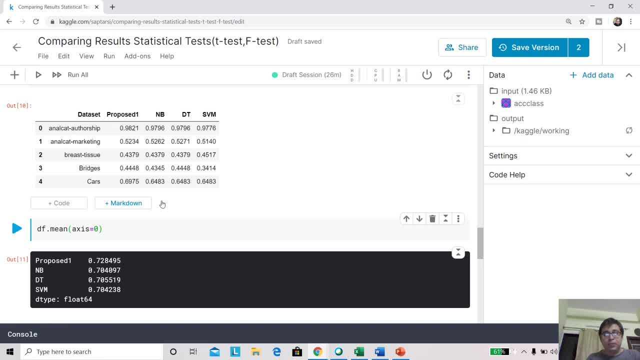 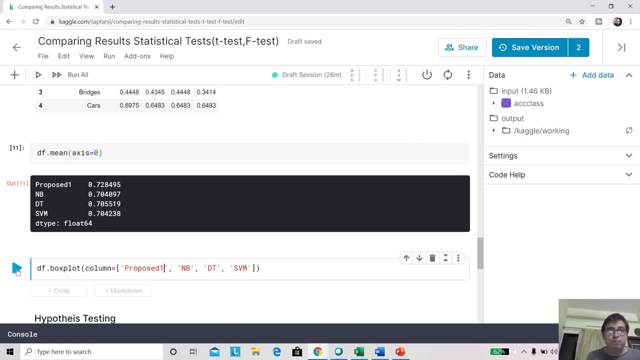 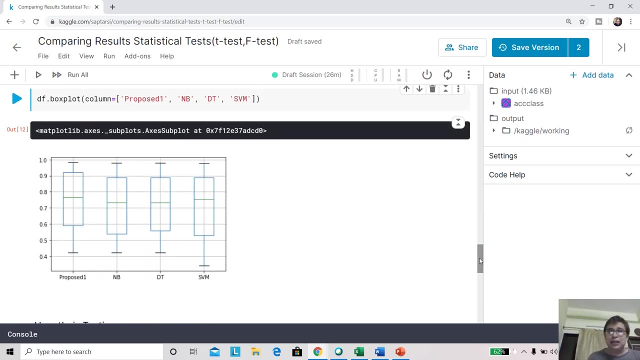 statistically significant. okay, so to satisfy them, maybe you can resort to a visualization. so let's take a box, plot and and plot the accuracy of each one of these methods. okay, so when we plot them, we still see that the mean of this method is indeed, you know, uh, indeed little. 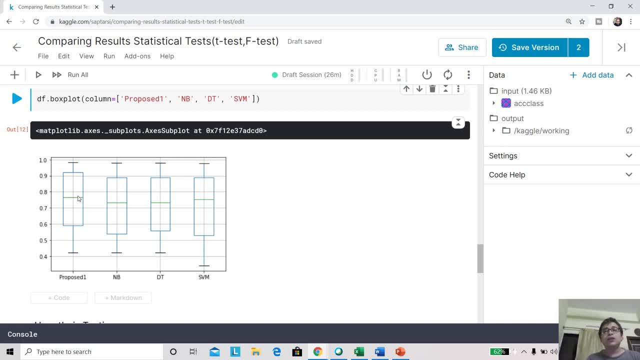 higher. so you know, box plot, this is the mean, right. so the mean is indeed, you know, above the other methods, and variance is comparable. okay, but still, statisticians or reviewers will not be satisfied, okay, so let's see how we can form the hypothesis testing from here. 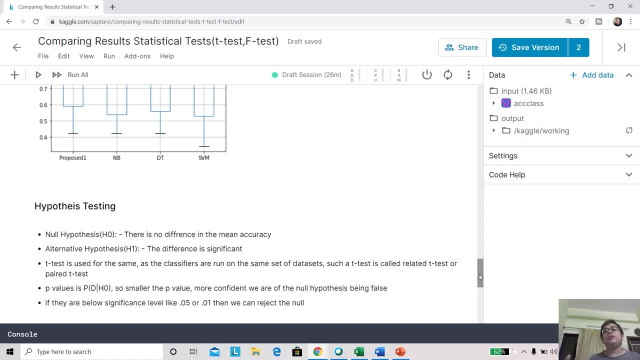 so your null hypothesis, you said, is that there is no difference between the mean accuracy. so you know, uh, first we are going to do a pairwise testing, so we are just going to compare two algorithms. so we are assuming that there is no difference, or the difference, even if it is there, it is not statistically significant. okay, so that is your. 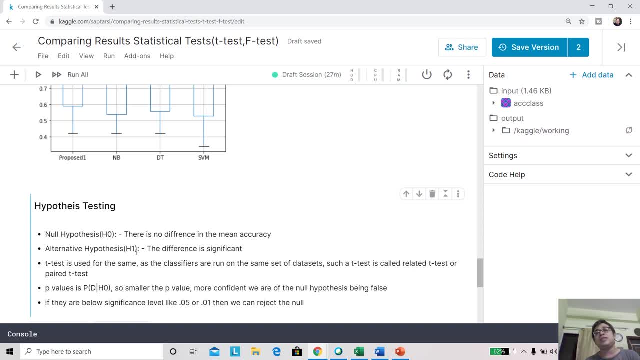 null hypothesis: there is no difference and alternative hypothesis is: the difference is significant. so what we'll do is: we'll do it. we'll run a t test. okay, and as the classifiers are run on the same set of data sets, you call this t test as a related t test or paired tickets, okay. 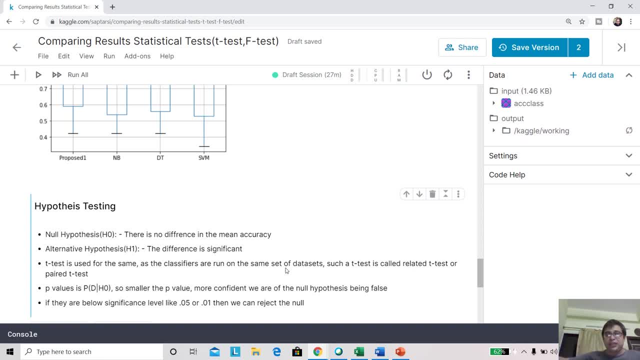 so if they were run on, you know different uh set of data sets these two algorithms. then you call it independent tickets. okay, and then, like all hypothesis testing, you find p value, which is nothing but probability of the data, given the null hypothesis. so smaller the p value you. 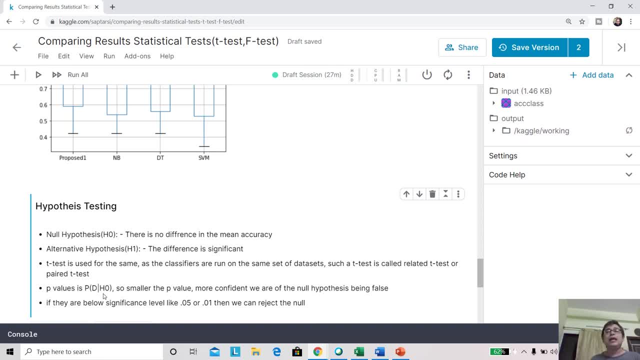 are more confident that the null hypothesis is false. that means that the difference in the mean accuracy is actually there, okay, and so you want your p value to be as small as possible. however, there is a significance level for the test, which is often set as point zero five. 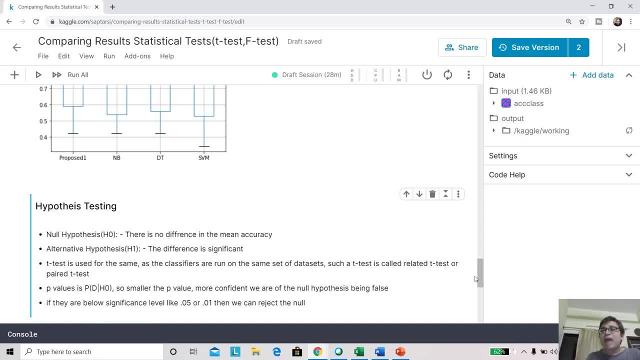 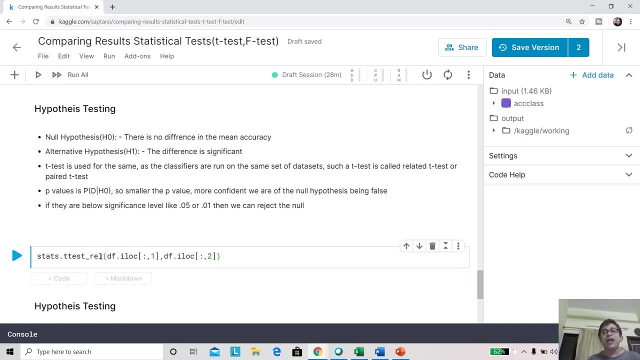 or 0.01.. So these are allowable level of p-value. So I can simply use this stats library and this ttest rel- rel means related and we are just testing the first two algorithms proposed with the next algorithm. So let me run this and if you see, it is giving me a statistic. 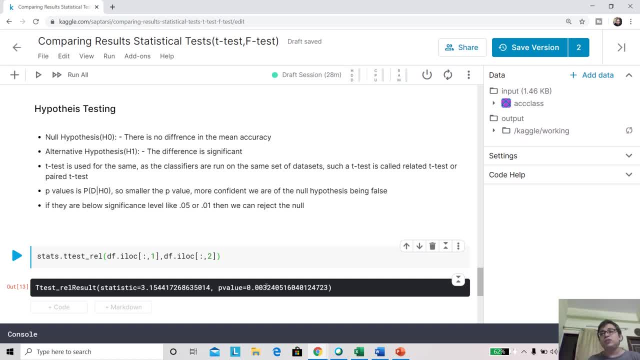 of 3.15 and a p-value of 0.03.. So even if you don't worry about this t-value, this p-value tells me that this is a very, very small value. So that means the probability of no difference, given the result that we have got, is very, very small. So we will reject the null hypothesis. 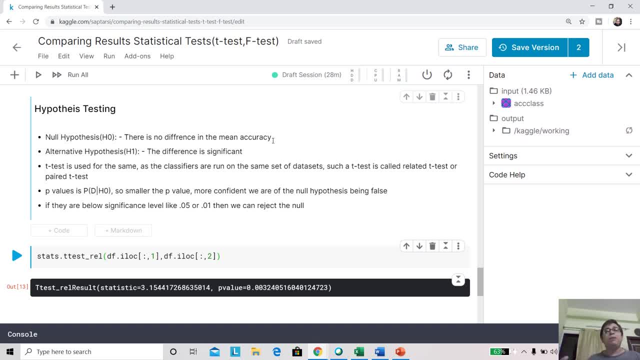 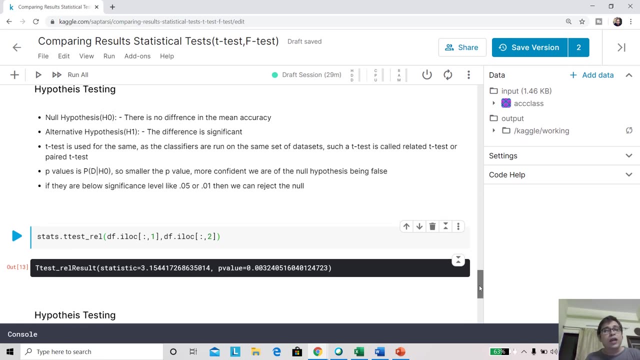 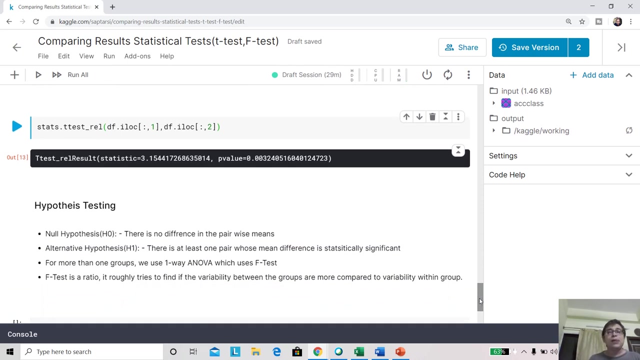 So this way you can actually set up your statistical test and show that your algorithm is statistically significant. So ttest can be applied only when we are doing a pairwise comparison. For a more involved test, What you can do is that you can go for a f-test. So what f-test does? firstly, it allows you. 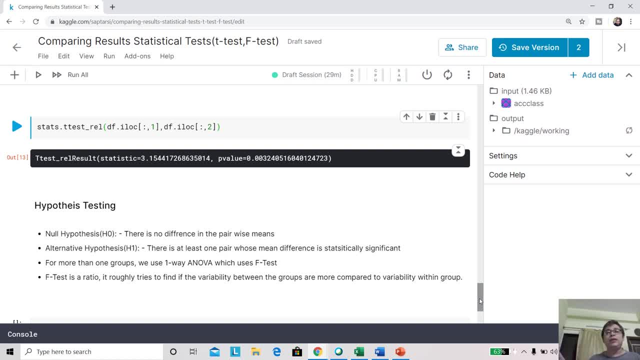 to compare mean of more than two groups. So null hypothesis is that there is no difference in the pairwise means. So if you have a, b, c, so a b is not different, b c is not different, c a is not different. And alternative hypothesis is that there is at least one pair whose mean 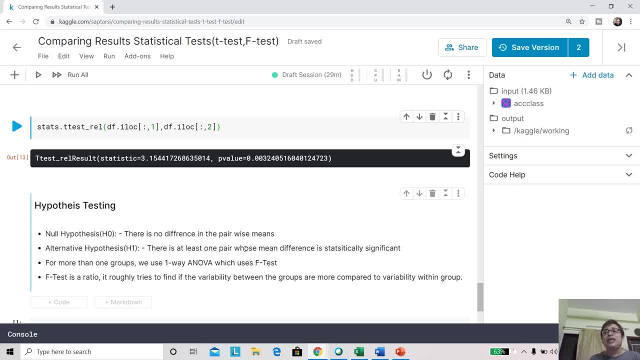 difference is statistically significant. So for that you use a f-test. Now, f-statistics is actually a ratio, So where you try to find out that whether the ratio of your inter-group variance and the within-group variance is high or not. So if f-value is high, that means that between the group your variance is high. 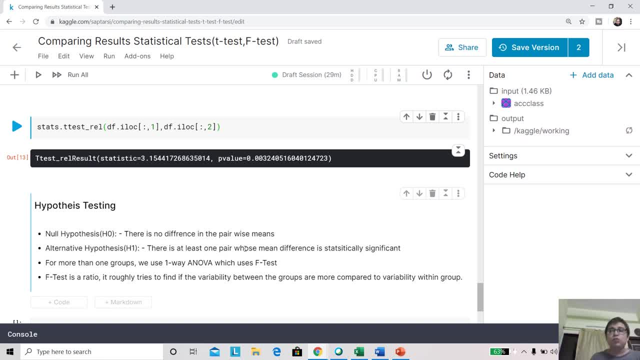 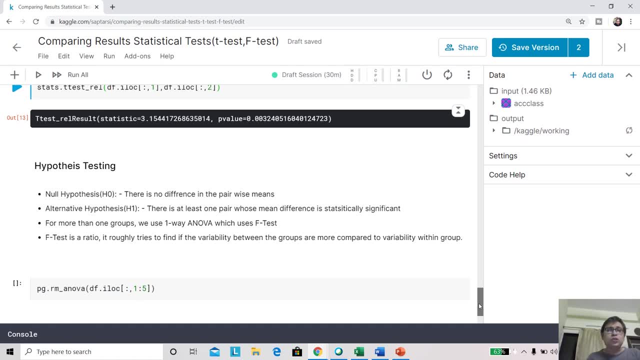 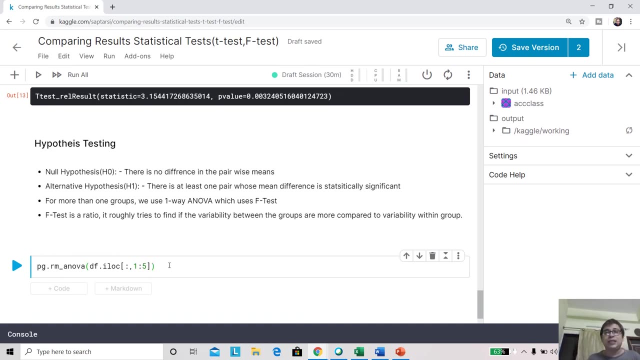 So if that value goes up, like for t-value, you know your probability of rejecting the null will also be high. So here also the test is very simple. So this is also as you are doing it on the same set of data sets. So this you call it as a repeated method, ANOVA, which is signified as R-M ANOVA. 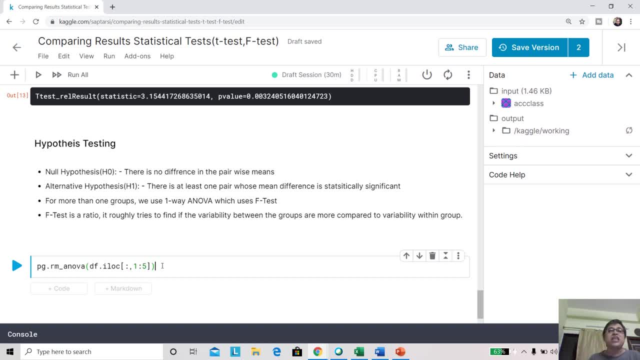 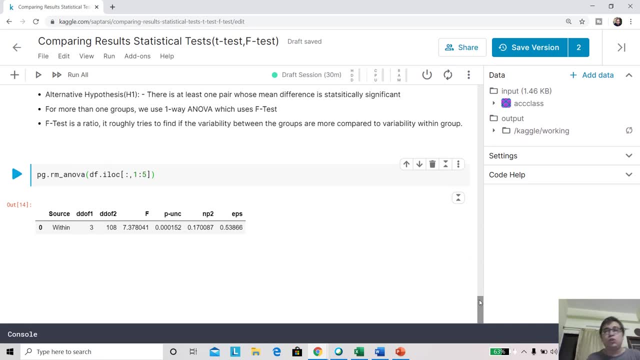 And here what we can do is we can run this on the entire results at the same time, And here it gives you some values. So important values are this: f-value and f-value. So if you want to run this on the entire results, 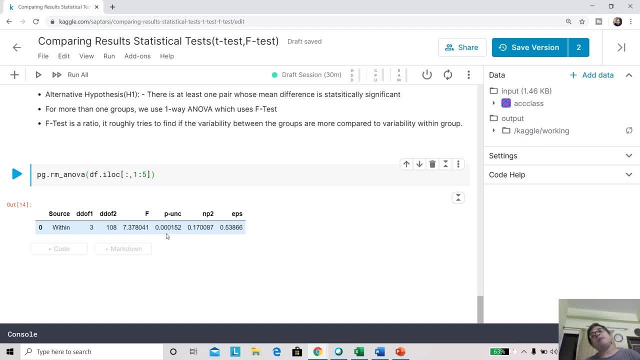 at the same time, And here it gives you some values. So important values are this f-value and this p-value. So you see again, p-value is very, very small. So you can conclude: the difference that you are getting is definitely statistically significant. However, please note that this f-test, or ANOVA,